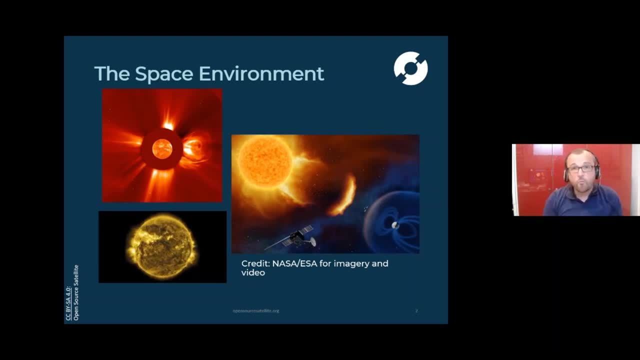 particles shoot out into space and they hit whatever is in their path. And the bad news is we are sometimes in that path. But the Earth has a defence mechanism. The defence is the Earth's magnetic field, which you can sort of see over here. The magnetic field of the Earth draws those 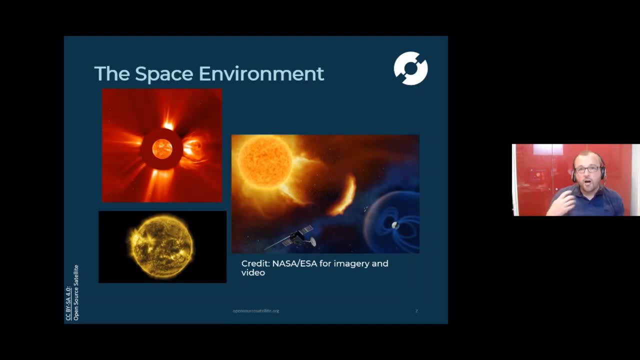 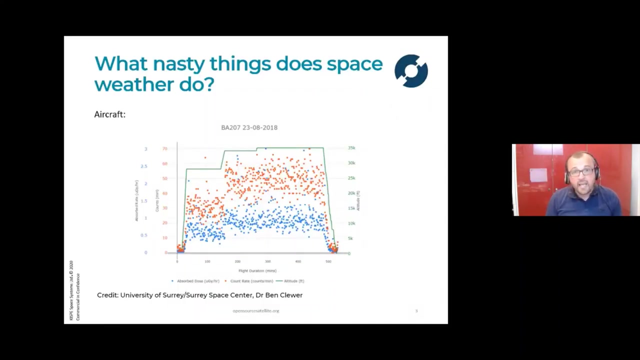 high energy particles away from harming us as people. But, as you can imagine, the higher you get out of the Earth's atmosphere, the more you see the effects of these high energy particles And in fact you can even see them in aircraft. And this is a study, the results of a study that 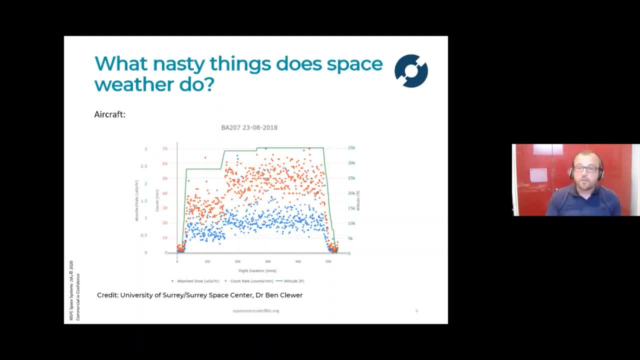 has been performed by the University of Surrey and my colleague, Dr Benjamin Kluwer, And here you can see basically what Ben is doing. He is giving people little boxes which have kind of radiation monitors in them. People take them onto their commercial air flights and they sit in the cabin and they fly around And all the time. 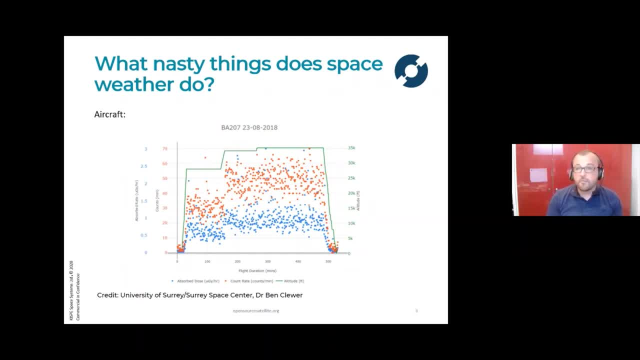 this thing is monitoring the amount of radiation dose seen within the aircraft And you can see here the results. So as you are on the ground waiting to take off, the radiation environment looks fairly sort of benign and not a lot of activity. And then, as you take, 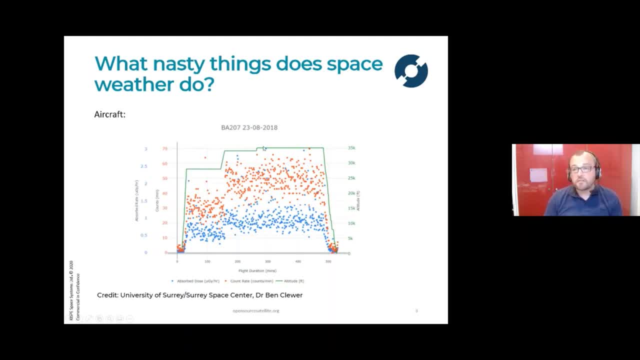 off and you go up into space, you can see that there's a lot of radiation And you can see that the altitude is now approaching 35,000 feet. You can see that the radiation dose increases And then it goes back down again at the end of the flight. And the interesting thing, it's not even just a function of altitude. latitude and other factors make a difference. So this is a flight from Dubai to London Heathrow And you can see here that, despite the fact that the altitude increases quite a bit again, up to sort of beyond 35,000 feet, you can see the radiation. 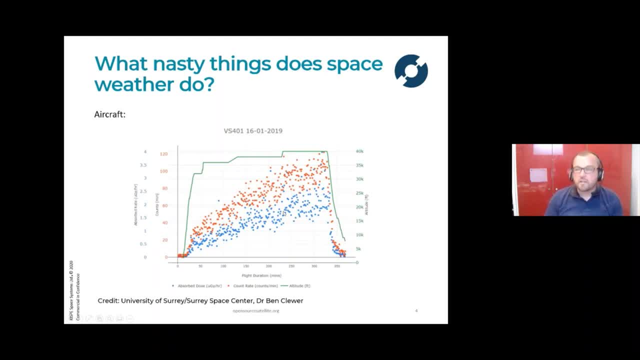 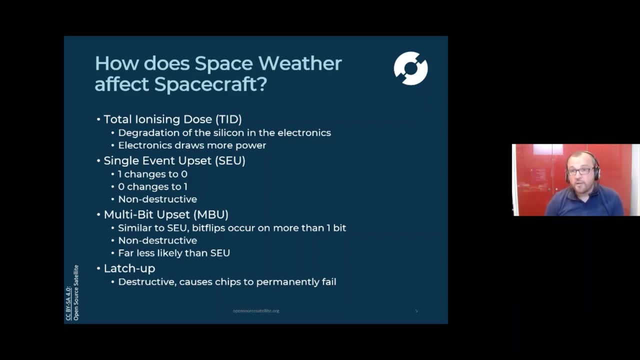 dose isn't really that bad until you get into the northern hemisphere. So, yeah, don't go there, I don't know. But what effect does this have on spacecraft? Well, there are a number of effects, because as you go out further from the Earth's atmosphere, the effects of the radiation, kind of 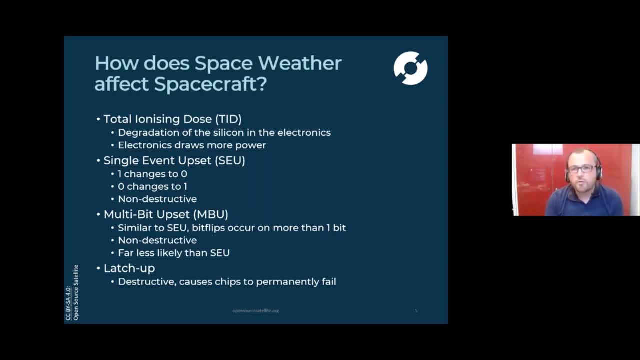 get worse. So there's an effect called total ionising dose And that's where you have these high energy particles causing gradual degradation to the silicon in the atmosphere. And that's where you have these high energy particles causing gradual degradation to the silicon in the atmosphere. 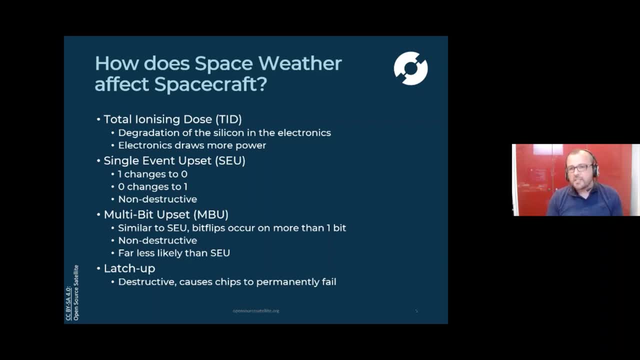 electronics within the spacecraft and what happens is that those electronic components, they start to draw more and more power over a period of time and it's kind of a slow process and, depending upon the technology and all sorts of things, the amount of shielding and stuff you can, you can see that. 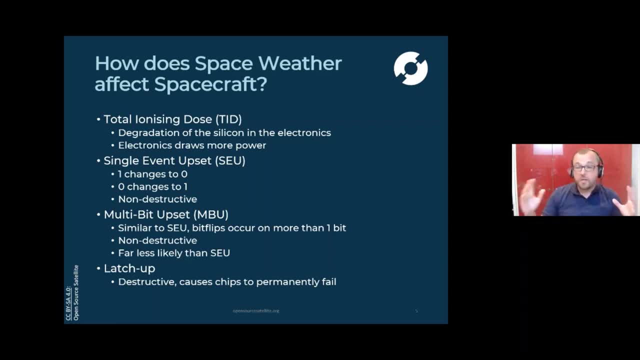 the electronics will draw too much power for the spacecraft to deliver, and if you know much about spacecraft design, you'll know that power is at a premium. we haven't got a power station next door. we get all of our solar power from solar panels, so it's very limited and- and this can be a problem- 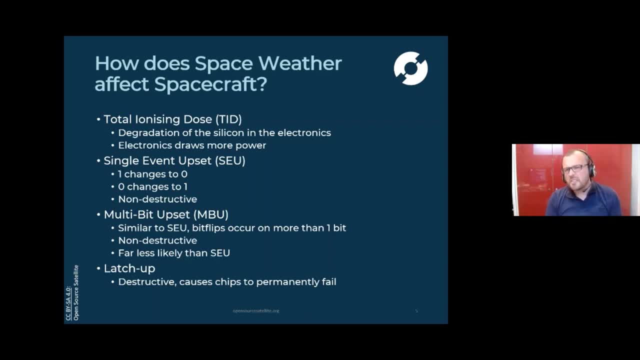 it can limit the life of a spacecraft. the next problem is kind of slightly more difficult to deal with in a way, and that's called a single event upset, and that's where these high energy particles actually hit the silicon and cause a one to become a zero or a zero to become a one. 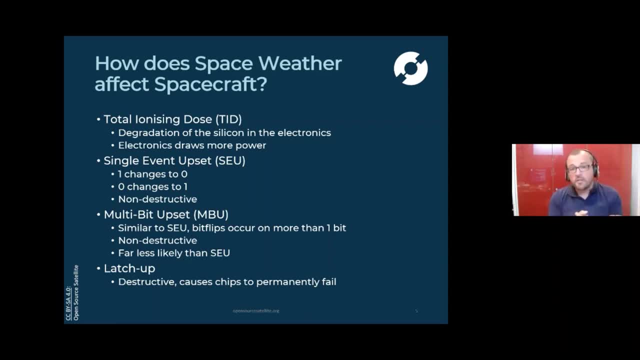 and if you know much about electronics then you'll know on computers, then you'll know that really the only things that computers understand are one and zero. you just put lots of them together and then you get something that's kind of a bit more intelligent. but what computers really cannot? 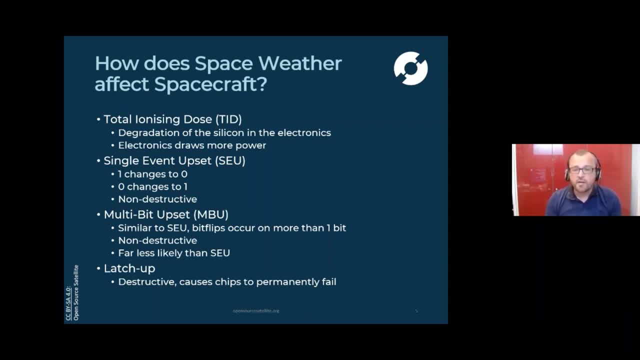 cope with is if you flip a one to a zero and a zero to a one when the computer isn't expecting it and the result of that is kind of a node. it depends where that happened in in the memory of the computer. it could have a disaster. 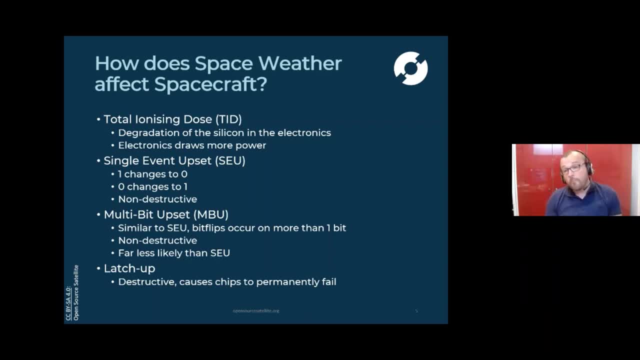 effect and it could cause the computer to crash, or it might just be something that doesn't really matter too much at all. it depends and it's difficult to predict. and then there's another effect called the multi-bit upset, which is basically the same as an seu or a single event. 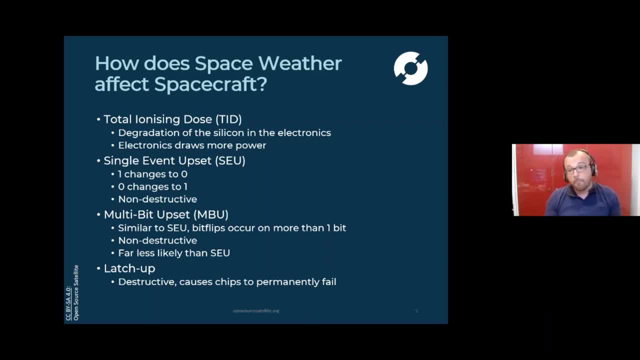 upset but it's where the uh bit flip occurs, on more than one bit it. but you know, both seus and and mbus are non-destructive. they don't cause any permanent damage to the silicon and they're far less an mbus and they're far less likely to cause an accident and they're far less likely to cause. 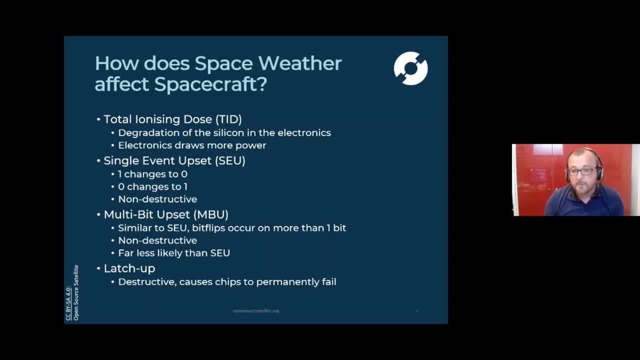 an accident and they're far less likely to cause an accident and they're far less likely to cause an mbu. a multi-bit upset is far less likely to happen than an seu. but the fourth effect is quite difficult to deal with and quite disastrous really: a latch up effect or a single event, latch up and 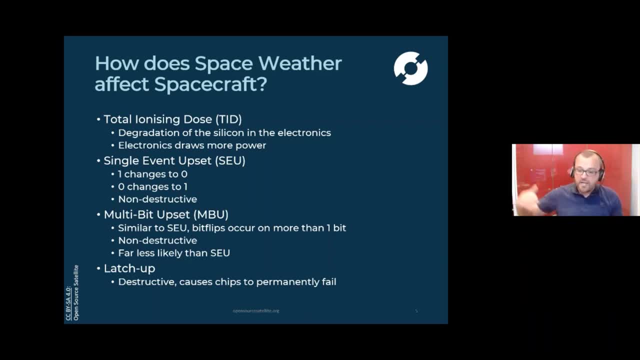 that's a destructive effect where it can be, and that's where um high energy particles hit certain parts of the silicon, causing a short across the power rail to ground uh and uh. you know that that means that the uh electronics starts to draw a lot, lot more. 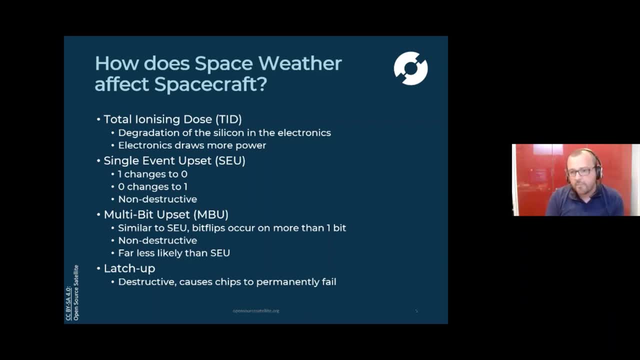 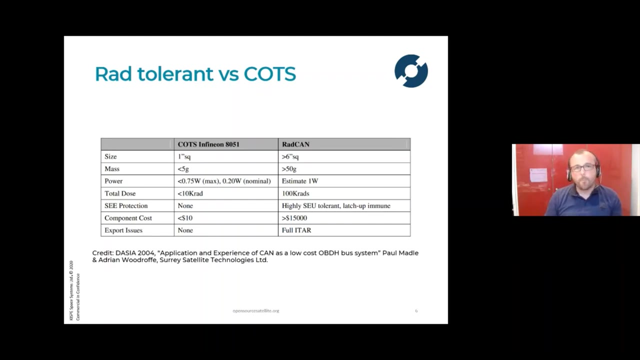 power and if that's there for um too long a period of time in under those conditions then it can cause a permanent failure of that piece of electronics and then it's really game over for that computer so difficult to deal with. so what is the space in the electronics industry done to kind of combat? 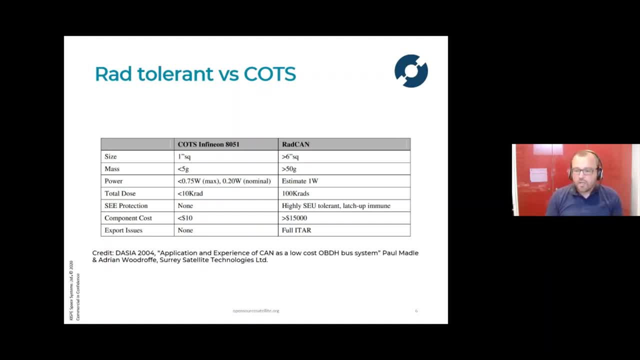 those kind of issues. well, um, early on, uh, with the sort of space industry that you know, the thought was right. let's make electronics that are robust against single event upsets and single event latch ups and total ionizing dose radiation. let's make something that's uh designed. 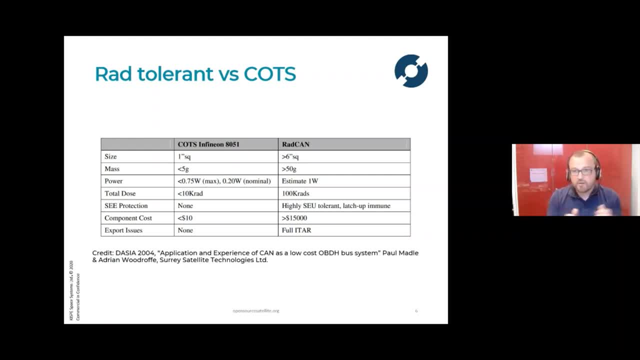 from the ground up to be resilient to that. so that's great. but what we discovered, uh, is that you know, or what we know, is that those technologies that employ that kind of technology, and they are generally, uh, quite sort of behind the equivalent commercial sort of uh technologies- 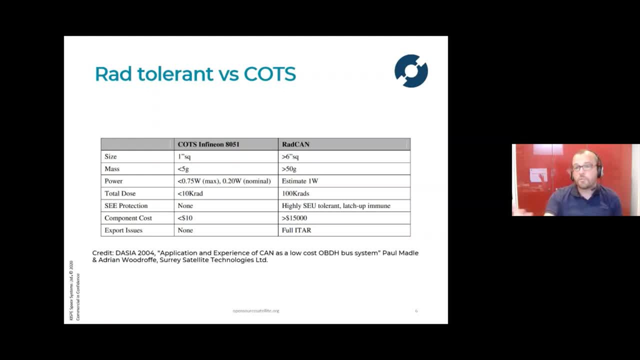 that you might find in your mobile phone or in your car or in your washing machine. and so companies a bit like um surrey, satellite technologies, they decided right, well, let's just kind of use commercial components, put them in space and see how they behave. and in fact they. 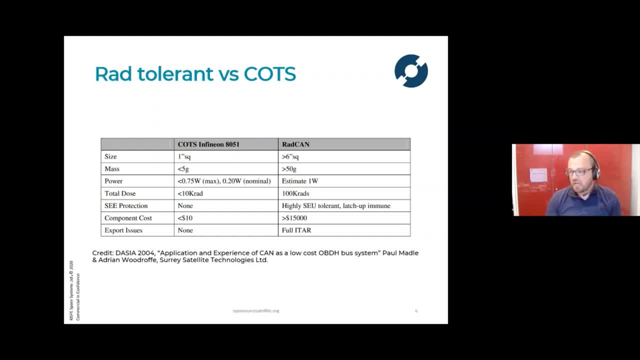 found that they behaved pretty well in benign sort of um radiation environments like that you find in low earth orbit, um, and in fact they started to employ uh commercial components. in particular, they used extensively uh an 8051 microcontroller, uh, but uh produced by infinian and uh they used extensively across their spacecraft. it's a. 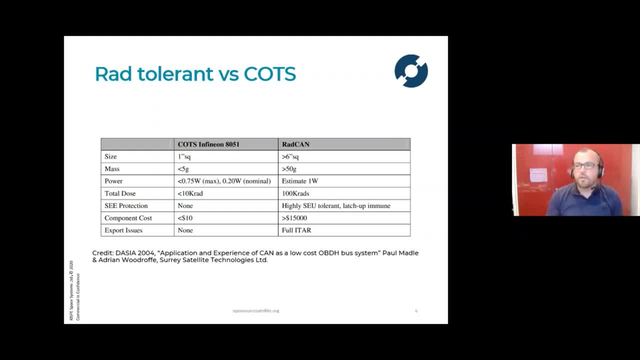 commercial component, um. but they needed then to do a mission which, uh, was going to be launched into a much higher orbit, and so its radiation environment, the radiation it would see, would be a lot more kind of a harsh environment. so they decided, let's make a functionally equivalent um computer. but 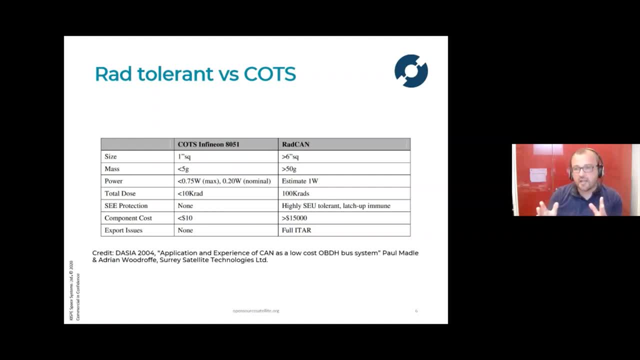 it's going to be radiation hardened and and so you can see that it's going to be a lot more expensive. and so you can see here the difference that you know making that decision makes, because the area of the electronics was a lot higher than the um. the mass was much higher. 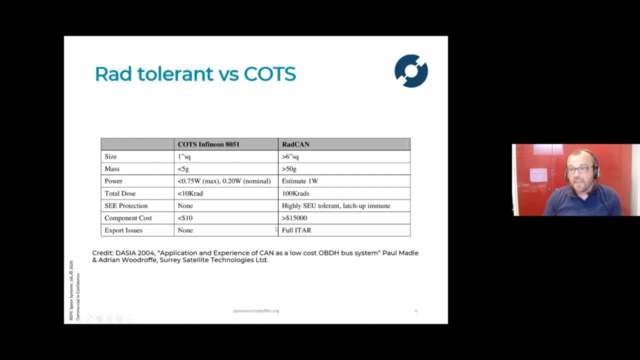 the component cost was gastronomically higher and then also the components that we used were american, so they came under full itar export regulation, which means that there's a lot more administration in trying to make use of these components. so what are we trying to do at um? 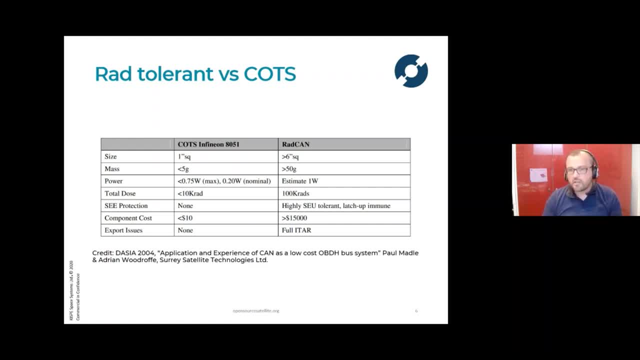 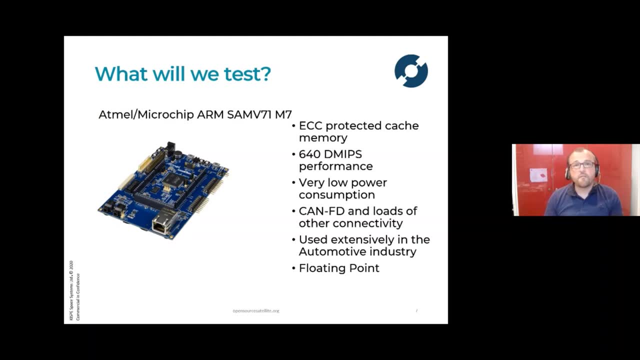 on the open source satellite project, we are trying to use um commercial components and we're going to test them. we're going to test them in representative environments to check how well they survive um, those, um, those four effects. and so we do, we've made, we've gone about sort of selecting some of the latest technologies. 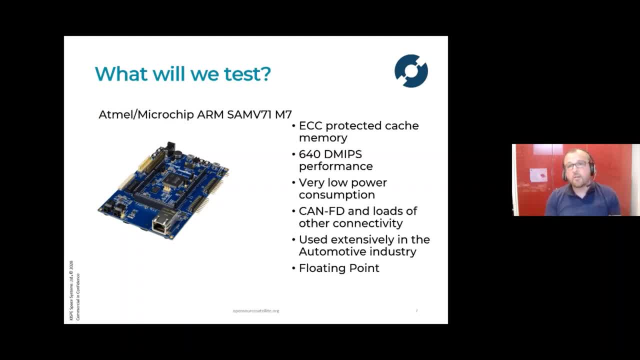 and we've gone extensively actually, with arm uh technology. uh, arm technology is used all over the world. it's used in your mobile phone, it's used, well, in pretty much all mobile phones on the globe. so you know, there's a lot of them, you know, as you know. so, um, why are they? why have we chosen? 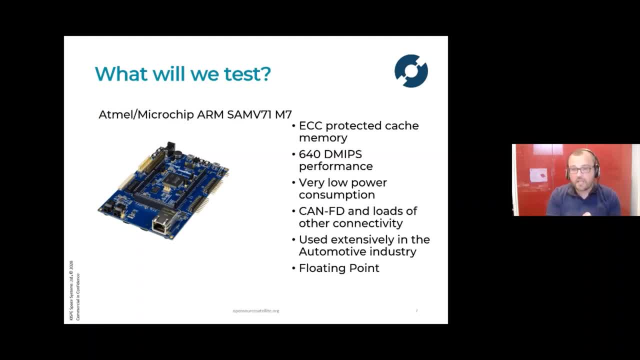 them well, because, because they're- they're used very, very frequently. um, there's not a lot of bugs inside them, because so many people are using them, and there are lots of open source tools to support the development of software that runs on them. uh, so that kind of suits our open source stuff. 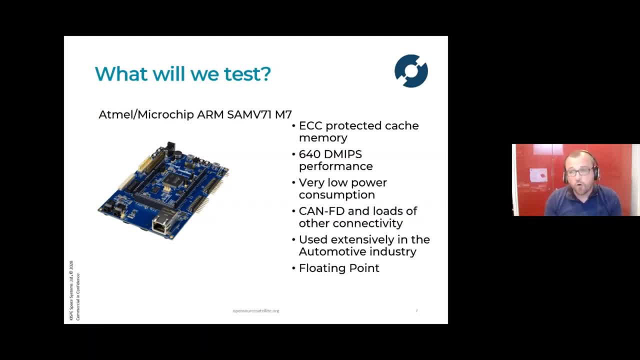 they're also well very high performance per watt of power and, as i said, you know, in space we're really worried about power consumption because there's not a lot of power to play with, and so these microprocessors are famed for having a low power consumption because they make use of a reduced instruction set. 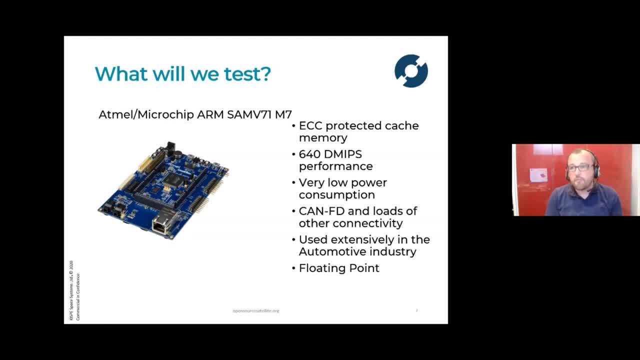 so we've chosen the atmel or microchip sam v71 uh arm microcontroller. it's a high-end microcontroller using an arm m7 cortex core and it's got. it performs 640 million instructions per second. um, it's got lots of connectivity and stuff and it also has a floating point unit. 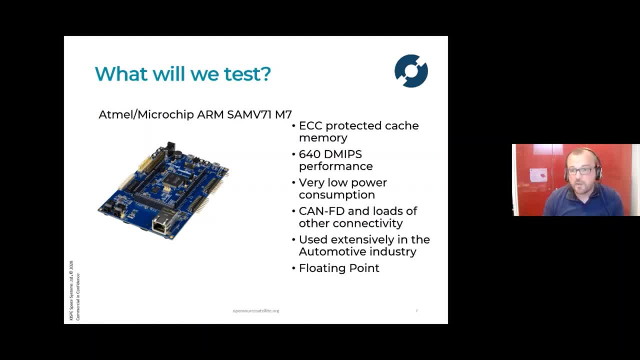 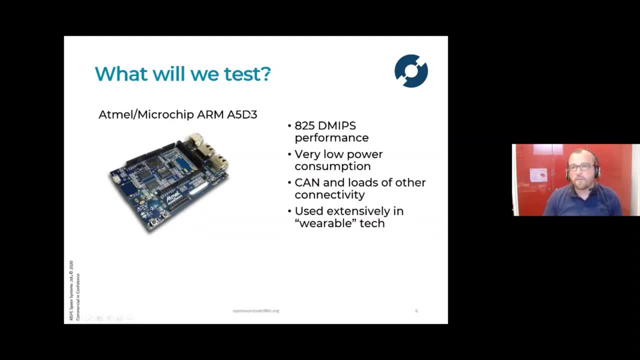 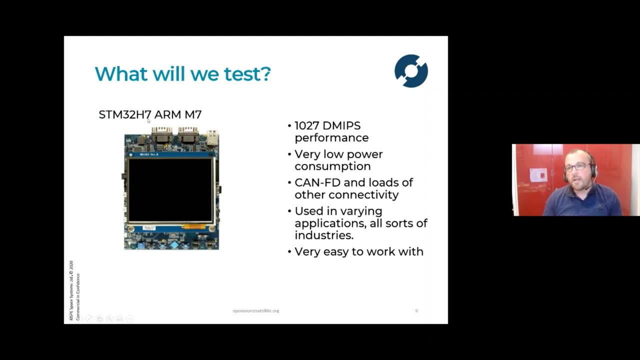 which is handy for doing maths, to ensure that the spacecraft stays in space. and for the same kind of reason, we've selected some other, uh um, micro processors. an arm, a5d3, again atmel microchip, one from st microelectronics. uh, an arm, another arm, cortex m7, so it's the stm32h7 and this one.